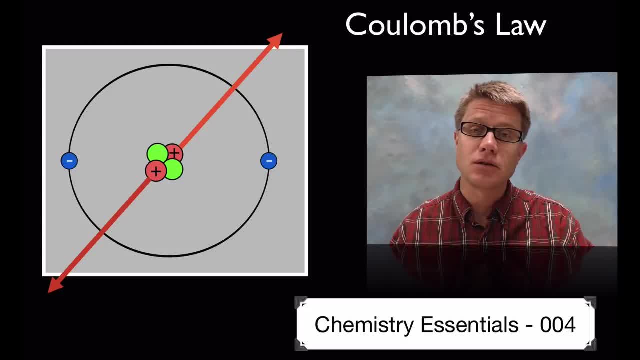 protons. And that's because, according to Coulomb's Law, as those charges get closer and closer and closer, then the forces get larger and larger and larger, And so it's sometimes referred to as the inverse square rule. And so let's get to Coulomb's Law. And why is it important? 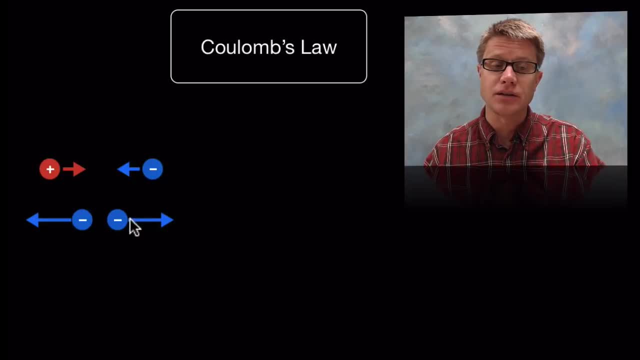 Well, again, it shows us that positive and negative attract, And it also tells us that if we have two like charges, they're going to repel, But the closer they get, the bigger that charge is going to be. And so Coulomb's Law tells us, the force between charged particles is proportional to their 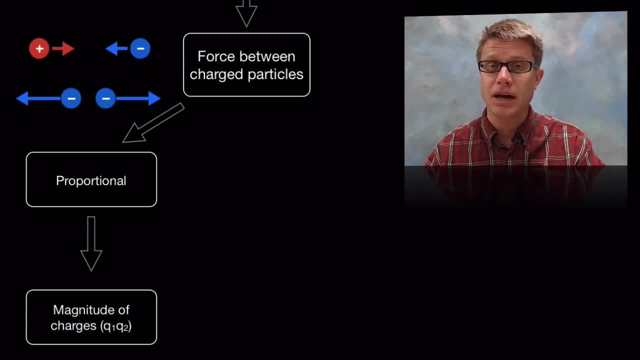 charges. So all you do is just multiply the two charges and that's going to give you the magnitude. It also tells us that it's inversely proportional to the square of their radius, In other words, how far they are apart. So if things are far apart, it's going to be less. 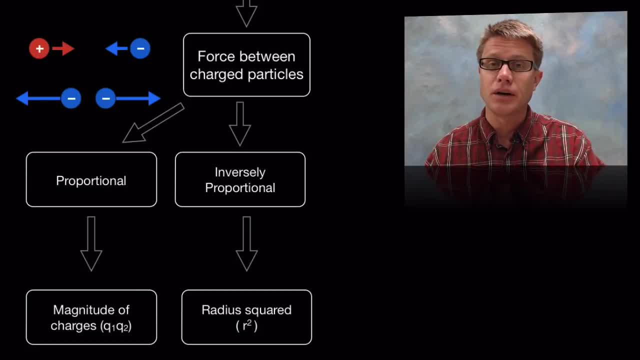 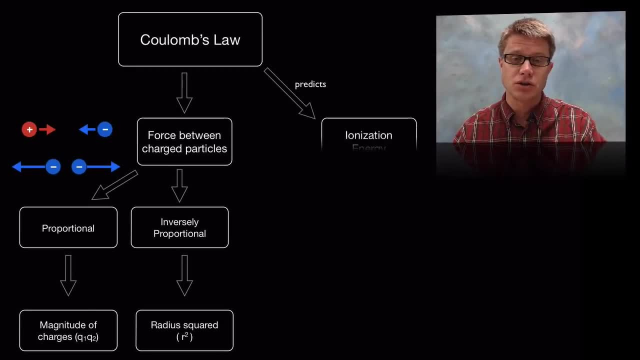 charge. As they get closer and closer and closer, that charge is going to get greater. It's very similar to the gravitational Newton's Law of universal gravitation. This just deals on the small level with charges. Now in chemistry it's important because we can use Coulomb's Law to predict ionization. 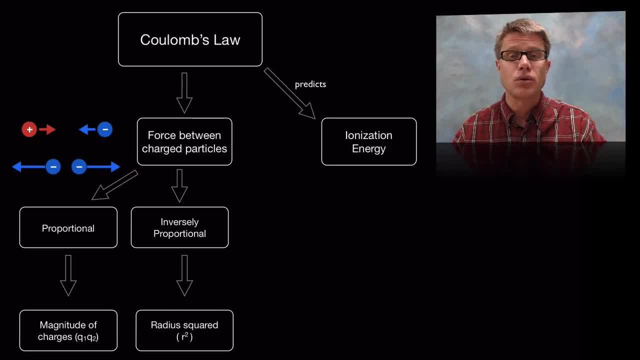 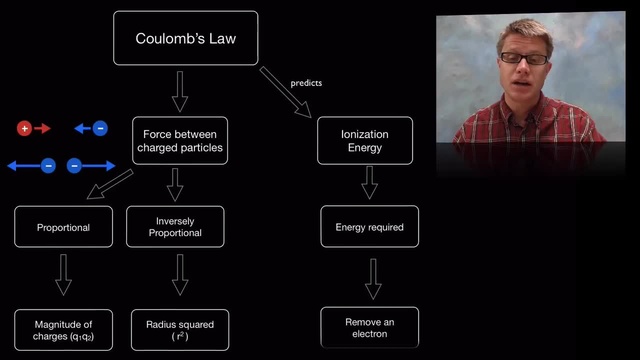 energy, Ionization. energy is the amount of energy that is required to create an ion. And so what's an ion? It's when you're either losing or gaining an electron, And so ionization is the energy required to remove an electron, And in chemistry, in science, we can actually 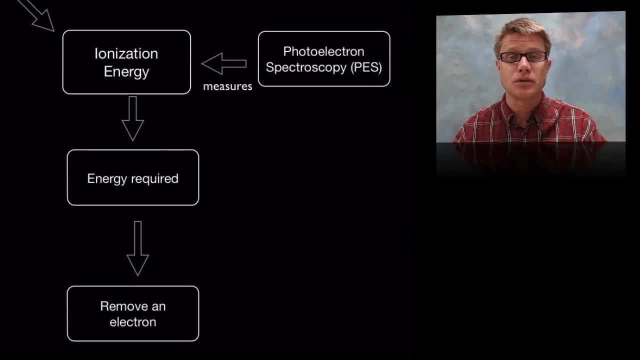 measure ionization energy using something called photo-electron spectroscopy or PES. Now, that seems confusing, but it's actually a really simple concept and has huge implications when it comes to understanding what an atom actually looks like. So we can use the data to predict the shell structure. So how do we know that we have these shells and orbitals? 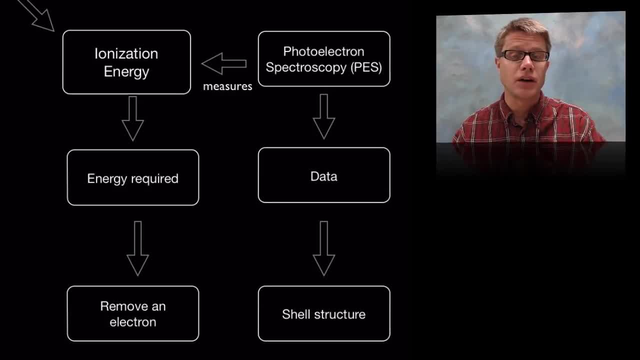 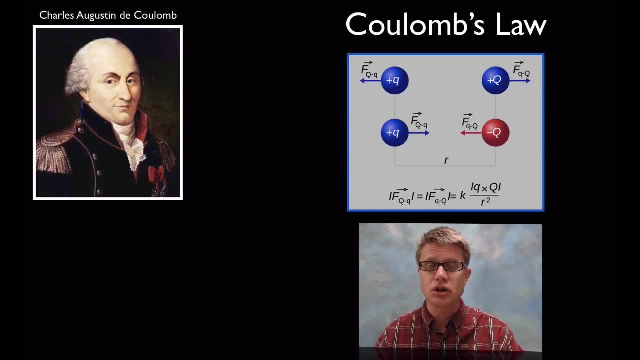 A lot of that is predicted through Coulomb's law, but it's also verified through PES. So who was Coulomb? He was a French physicist and what he was doing was studying charges. A lot of people thought there was some law that could be applied to charges, and he was. 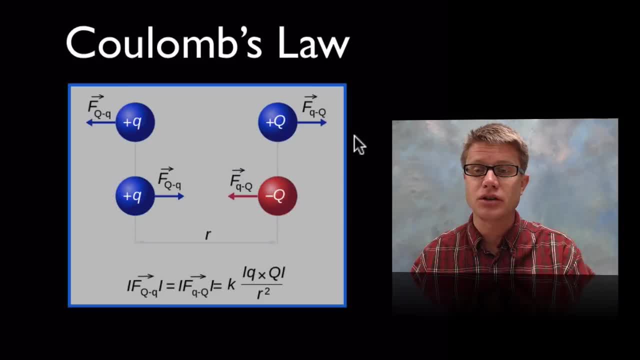 the first one to really quantify that. So essentially, if we have two like charges, they repel, And if we have two unlike charges there's going to be an attraction. And here's the equation right here. You have a Coulomb's coefficient and then we're going to have multiplying. 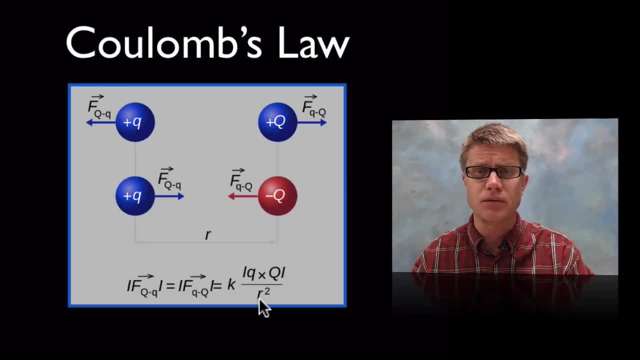 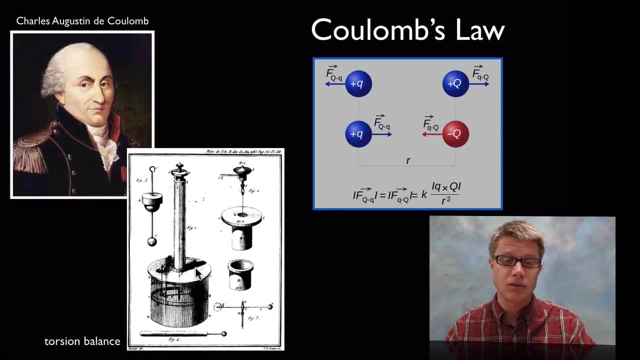 the charges, and then we're going to take the radius squared. Now, how did he discover this? Before we had electronics and even electricity had really been discovered? he used something called a torsion balance, And this is one of his sketches of a torsion balance, And 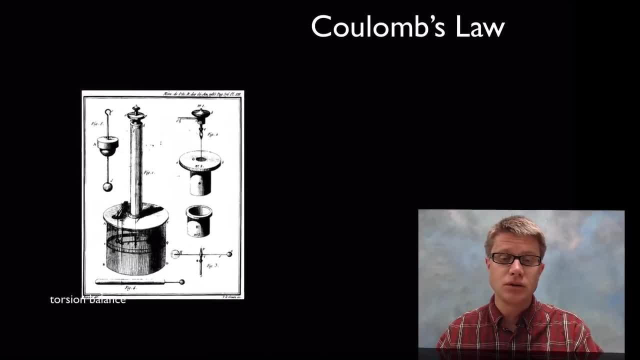 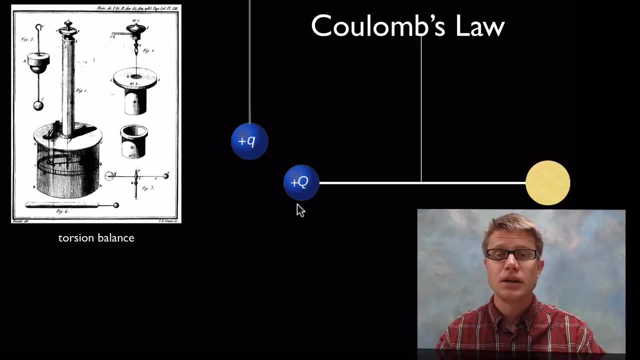 torsion balance. it looks a little complex, but it's really simple. All he would do is he would take a sphere and he would charge that sphere, And so we're talking about electrical, static electrical energy, And so that was suspended by a fiber all the way down here. 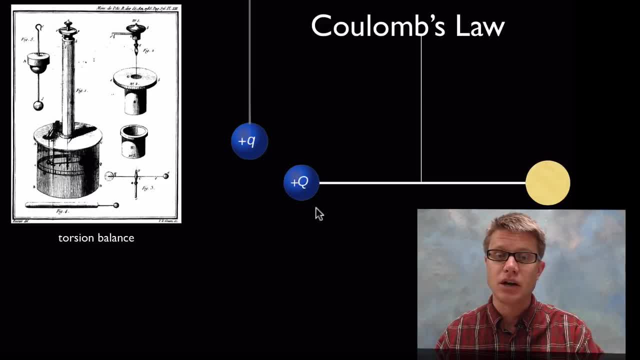 in the torsion balance. So he would give this a positive charge And he would give this a positive charge as well. And so if we have two like charges, what's going to happen when I bring this one? you can see it right here as I bring this closer. what's it going to? 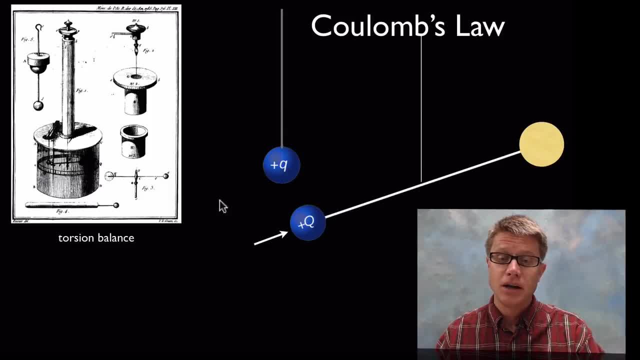 do? You can see it's going to go up and down. You can see it's going to go up and down. You can see that it's going to push it away, It's going to repel And so it would twist this fiber and he could measure it. You can kind of see the scale on the side He could. 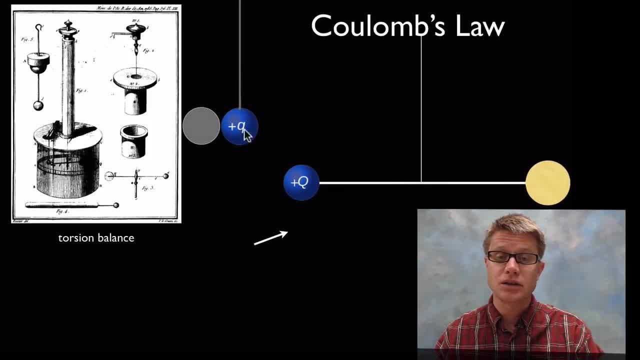 measure how far it went. He would then move it away and he would touch this sphere to another sphere that didn't have a charge, And what it would do is it would transfer half of its charge to that uncharged sphere. He would then bring it back again and it wouldn't. 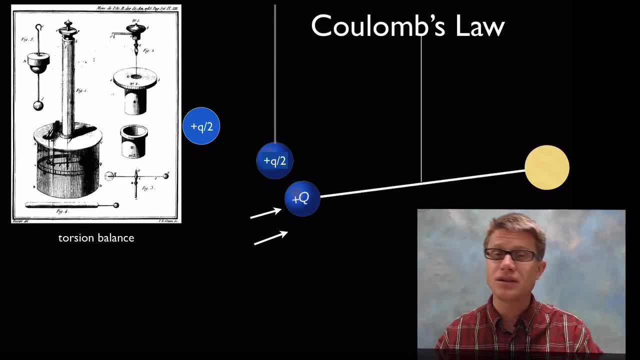 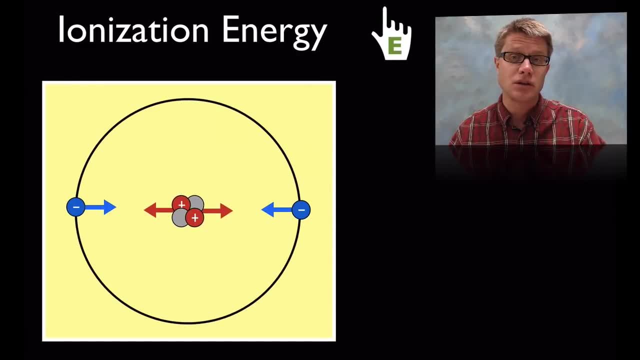 move as far, And so he was able to quantify Coulomb's law using a not super sophisticated torsion balance. And so why is this important? in chemistry, We can use it to measure the energy. We can use it to measure ionization energy. And so what's ionization energy? again, 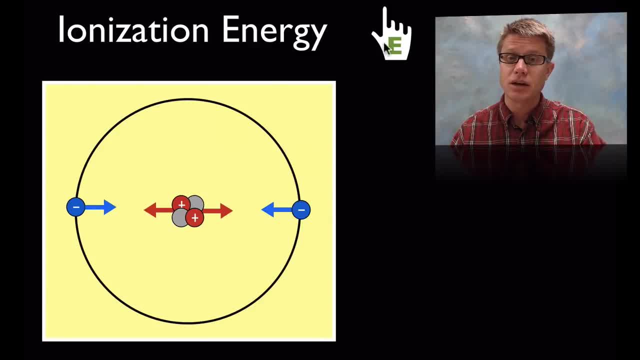 It's the amount of energy required to remove an electron. So think of it as just a little hand that has to come in and grab this electron and pull it off. So that's the ionization energy, And so it's going to depend on Coulomb's law how big that ionization energy is going. 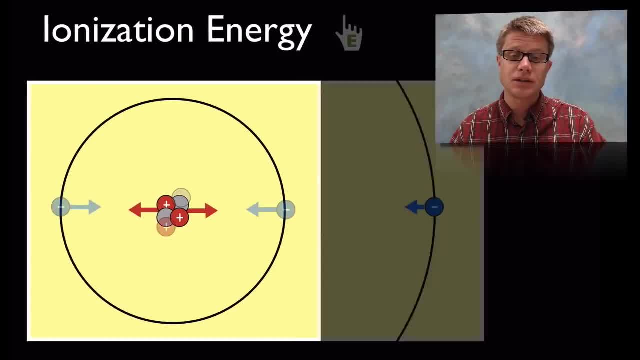 to be, Because that proton wants to hold it in place. And so let's say we were to look at something that's a little larger. So this is lithium, And so lithium is going to be the amount of energy that's going to be required to remove an electron, And so we're going. 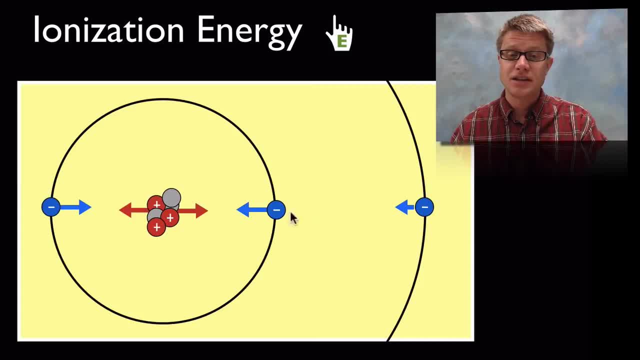 to have this outer electron out here, And since the distance is greater, in other words that radius is larger, you're going to require a smaller amount of ionization energy to pull it off. And so that Nobel Prize was awarded to Albert Einstein for his discovery of the 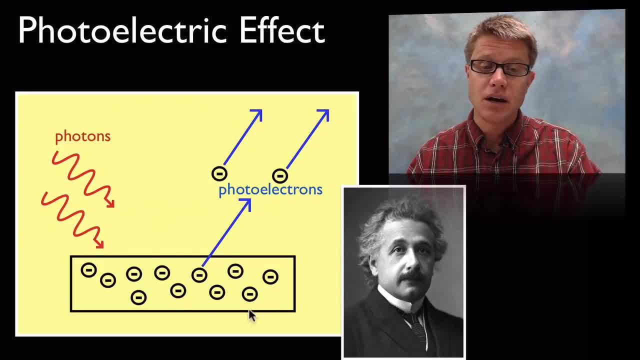 photoelectric effect, And what that means is, if you hit metal with photons or hit metal with light, what it will do is it will eject these electrons and we call those photoelectrons, And so hold on to this electron, And if it doesn't get there, we're going to have this: 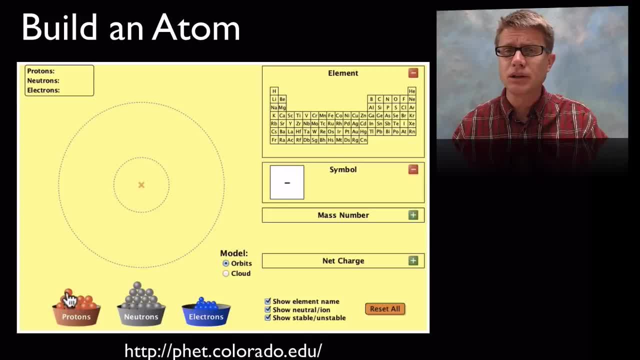 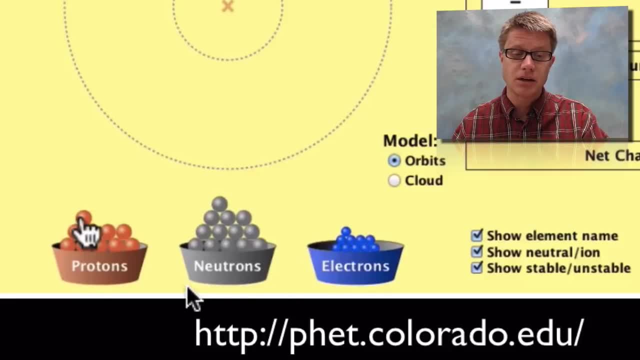 hold on to that idea. It's going to become really important in just a second. But let's build an atom for a second. And this is a simulation from PHET. What you can do: you could go to the website right down here. What you can do is you can just start dragging. 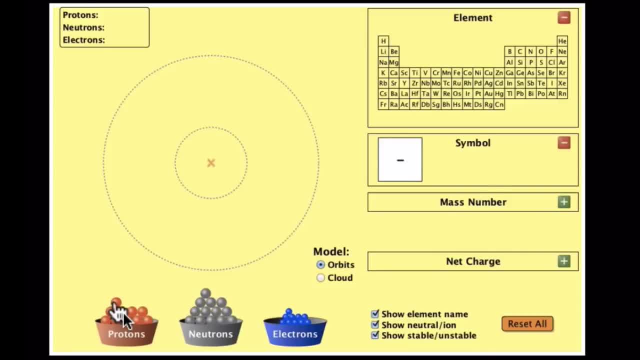 things in and then it will actually build that atom for you. So let's do that. So let's say I drag a proton in, I've now created hydrogen. You can see on the periodic table that's going to be H. It's got one atomic number. But let me just throw an electron in there. And where? 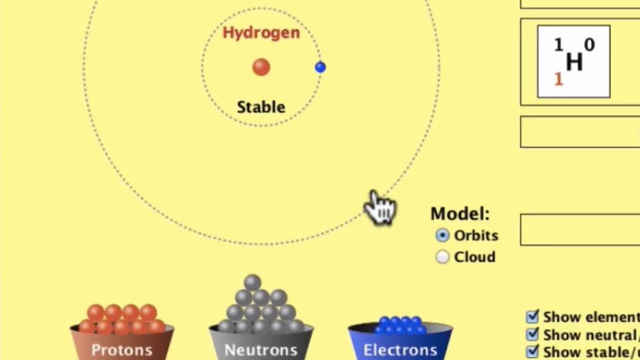 does it go? It goes right there. What's holding it in place is going to be Coulomb's law. They're opposite in charge, and so they're going to be held together. Well, what happens if I throw another proton in? Now we've got helium, But look how unstable it is. Why is 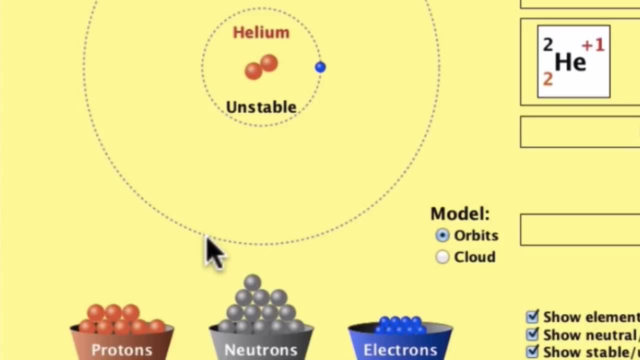 it so unstable? It's because those are like charges and so they want to repel each other. Luckily, if we and it would never exist like that. Luckily, if we add some neutrons to it, then we can stabilize it And so that's not going to decay. Now let's add another electron. 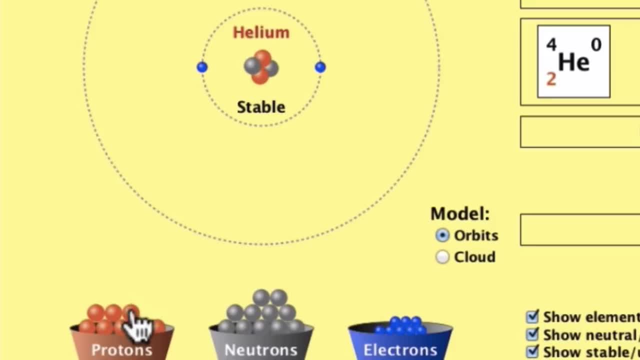 It's going to sit in this shell, And so we've got two electrons in this first shell. Let's make it from helium. let's move up. Make it a little bit of unstable lithium. We'll stabilize that with a neutron. Now let's 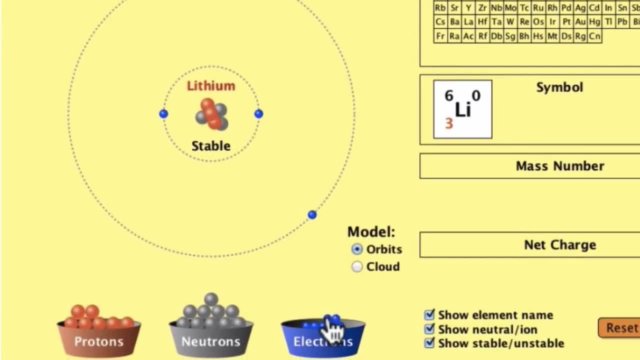 add another electron, What happens? Well, it sits right there. In other words, it's in the outer shell, And this is in the outer shell, And this is in the outer shell. So why is it that those first two electrons are going to be on the inside shell and the outer electrons? 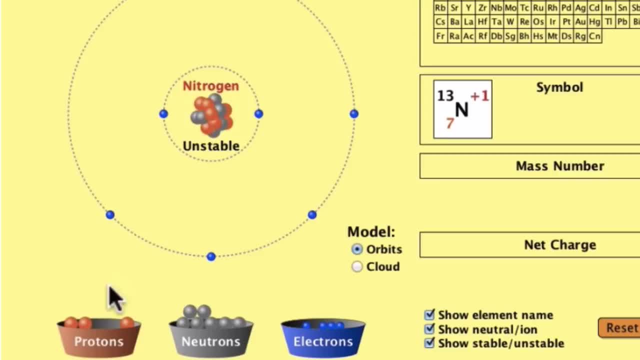 are going to carry, or, excuse me, those additional electrons that we add are all going to be thrown to the outside. That has to do with quantum mechanics and quantum physics, And so it's quantum numbers that are determining that. But how did physicists figure this out? How did chemists figure out that there's going? 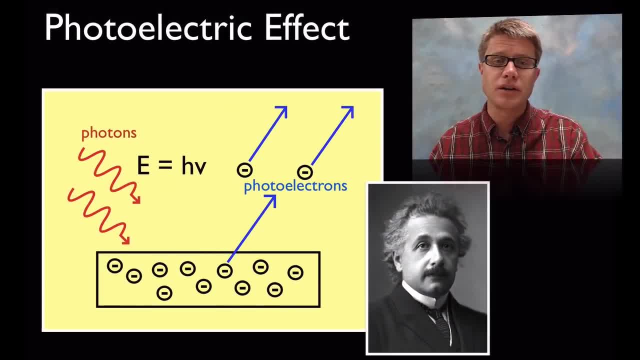 to be a 2 in the first, and then we're going to have 8 in the next and we're going to have all these orbitals. Well, we owe it to the photoelectric effect, And so, going back to that again, that's Einstein's theory that if you hit matter with light, it's going to 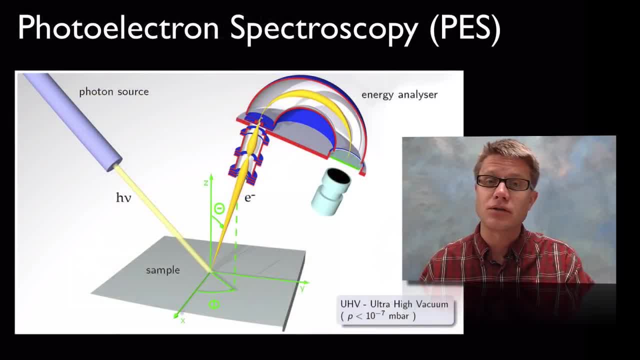 eject these photoelectrons, And so let me show you photoelectron spectroscopy. And so what is that? You basically have a photon source, You have a photon source, You have a photon source on one side, And so you're going to have a source of light on one side, And so 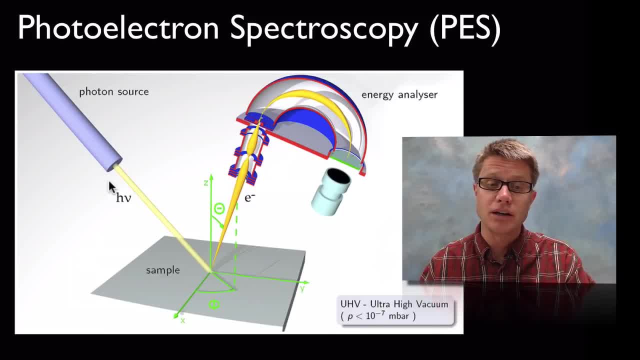 that could be infrared light, It could be UV light, It could be x-rays. The energy of those photons is determined according to the equation where energy is equal to hv, Where h is Planck's constant and v is going to be the frequency of the light. So basically, in 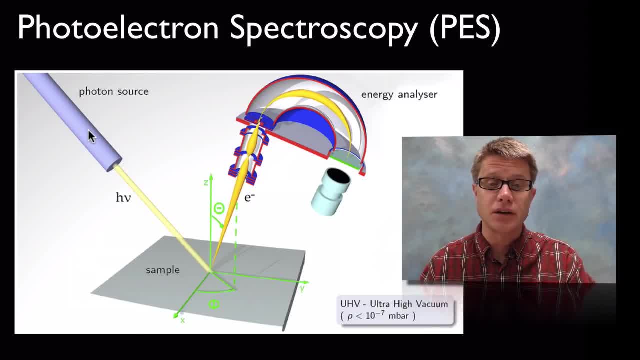 this machine you can vary the energy of those photons that are coming out. They'll strike the matter that you want to study that's sitting inside a vacuum And that's going to eject electrons, So photoelectrons, And those photoelectrons will be captured up above so we can measure. 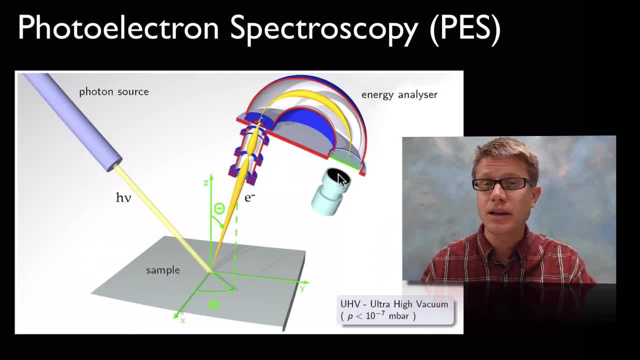 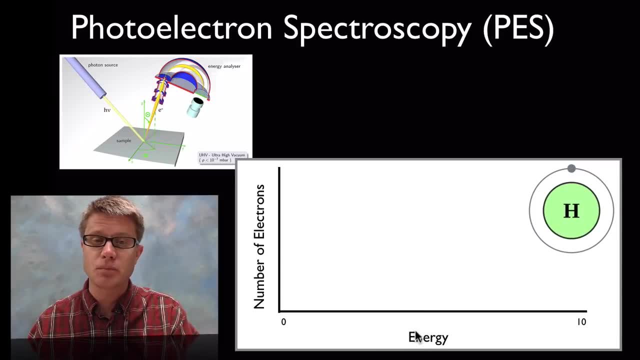 them, And so this is a pretty simple setup. What are you doing? You're hitting matter with light, and then you're measuring the electrons that come out of it. And so let's look at hydrogen. If we're looking at a sample of hydrogen, we're going to create a spectrum. 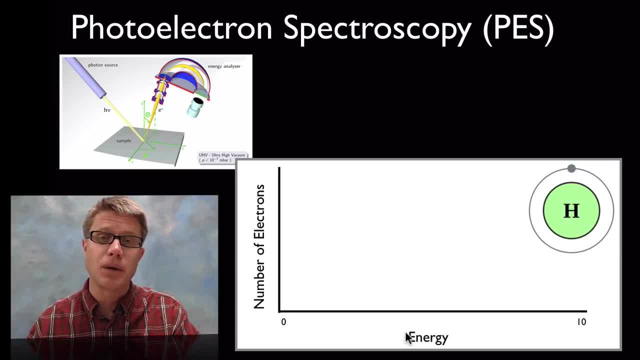 or a photoelectron spectrum, And so we're going to have energy across the bottom- That's the amount of energy that we're introducing with the light- And then we're going to have the number of electrons on the side. And so what happens when you turn on the machine? 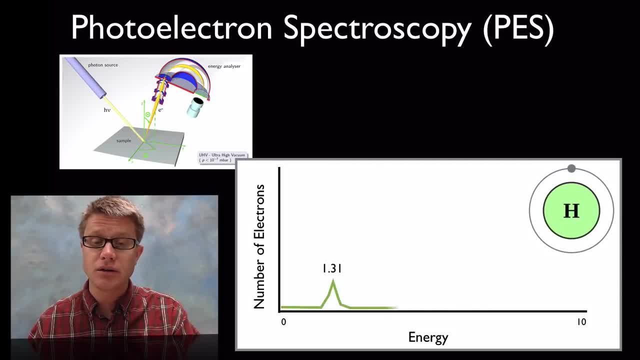 is, you can just vary the energy And eventually you'll hit a point where you get a bunch of electrons coming out. So why is that? Well, what we're doing is we're changing the amount of energy to the point where we hit ionization energy And then boom, we're going to release. 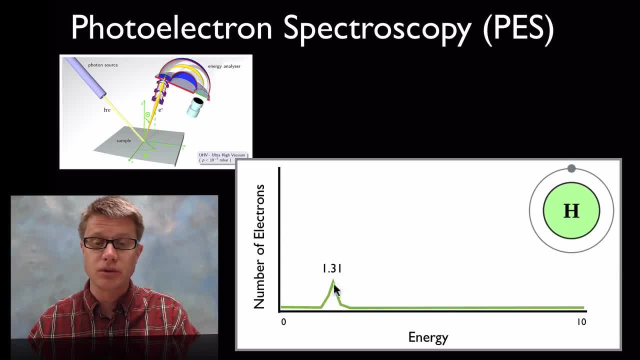 all of those electrons from hydrogen, And so we're going to get a peak at. we'll just call this 1.3 and think of it as an amount of energy. Now let's go to helium. What do you think that's going to look like? Well, helium has two protons on the inside, So it's 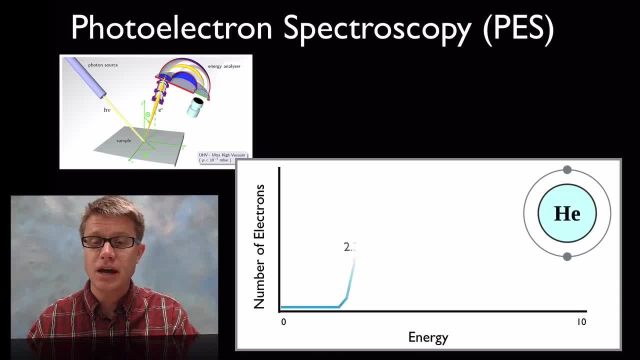 going to have a different amount of ionization energy, And so if we hit that with light, watch what happens. Okay, It's a different amount of energy. You can see that we need more energy to eject those electrons. But look how big the peak is. Now let's compare that back to hydrogen. Hydrogen had a peak. 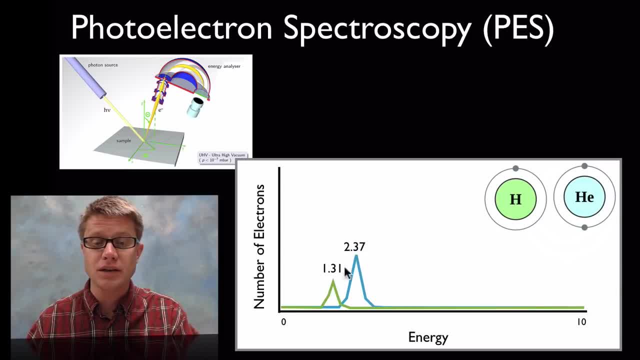 like this. Helium had a peak like that. Why is this twice as high as this one? It's because it has twice as many electrons. It's because we're ejecting two electrons when we tune that frequency to the right ionization energy. Okay, You think you got that. Let's go to.